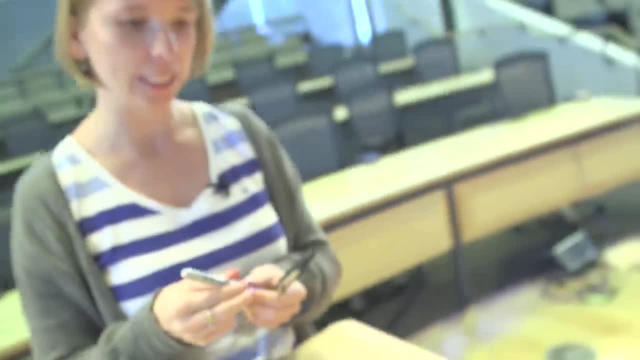 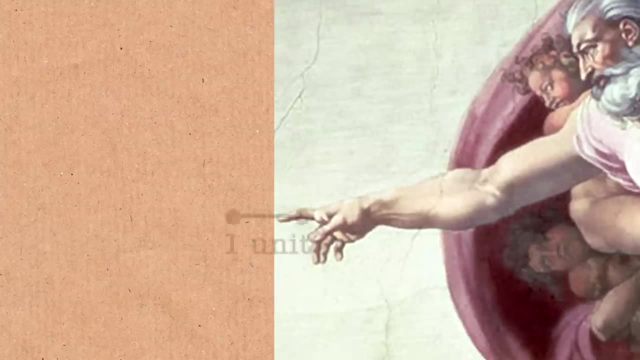 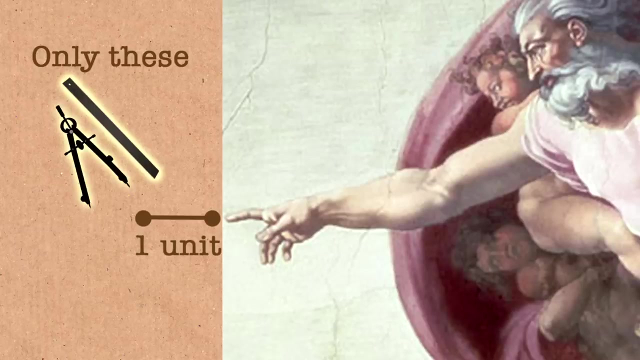 times. So one of the central questions that that people have been interested in for a long time is exactly what kind of lengths you can construct if you have a straight edge. So if you have a straight edge, you're given a line segment of one centimetre or one inch or one unit. Today, when you start, 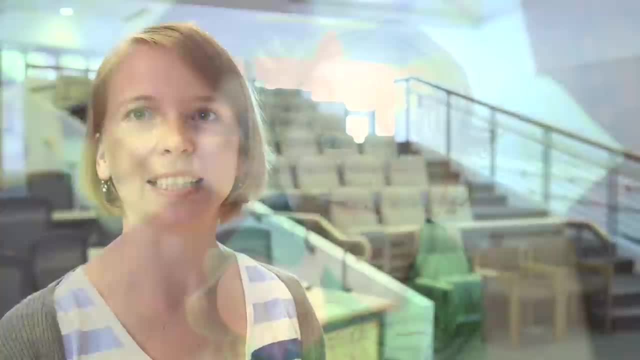 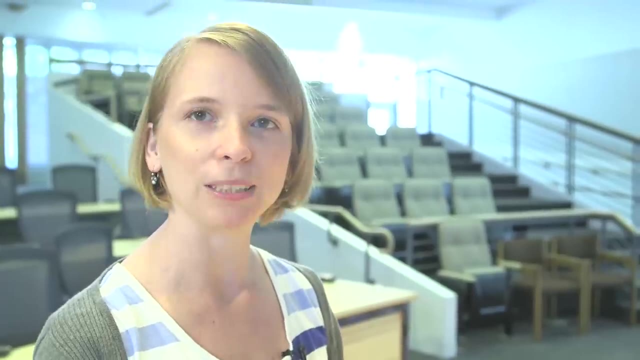 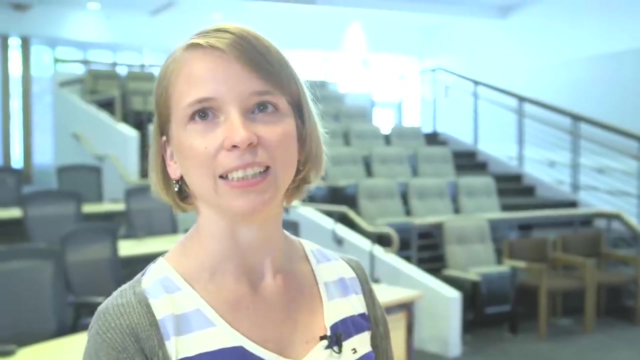 learning mathematics, even when you're two years old or three years old, you always start with numbers, But for Euclid and people in his time, it was the opposite. They thought about geometry as being the basis of everything, And they thought about shapes, points, lines, triangles being the 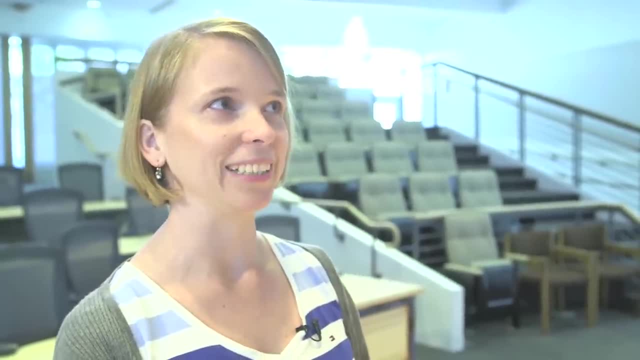 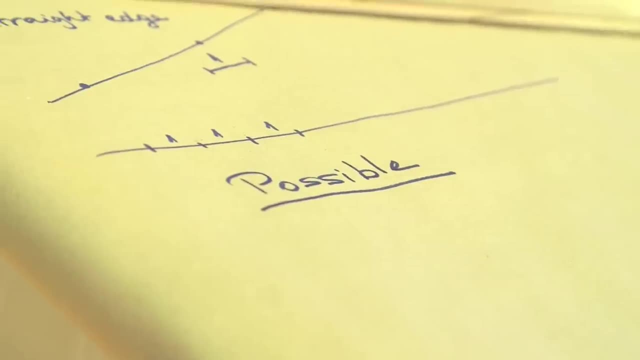 fundamental objects, And they thought of numbers only as something that arise from the geometry. So the questions that they naturally asked were a little bit different. So first I'll show you a few things that are possible. How about I give you a line? 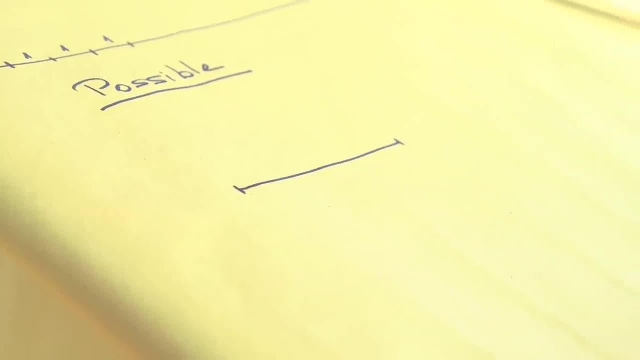 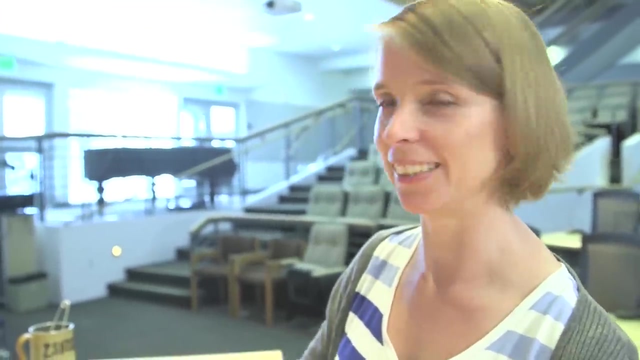 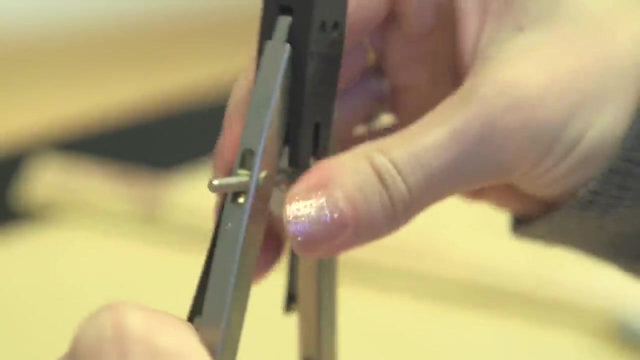 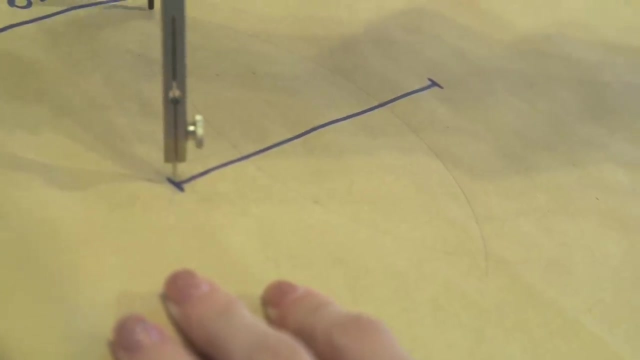 segment of some length and ask you to construct a perpendicular bisector, meaning a line that's perpendicular to this line segment and cuts it into equal pieces. I have to open this compass quite wide because I drew this long line segment, So I draw one circle arc, So I do two circle arcs. The important part is that the width of the 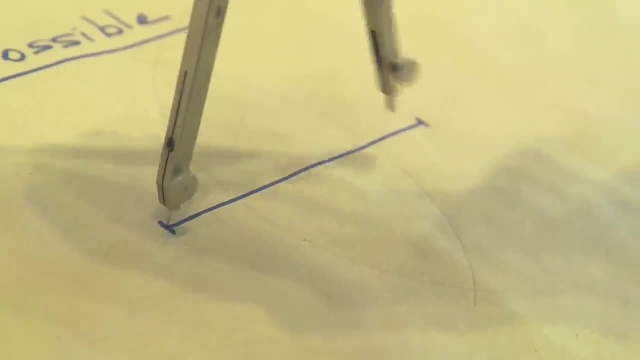 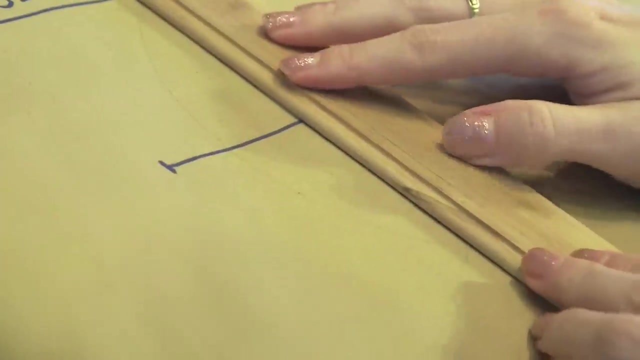 radius of the circle, so the width of the compass was the same when I do it from the left and when I do it from the right, And then take the straight edge and just connect the two points where those arcs intersected And they will. 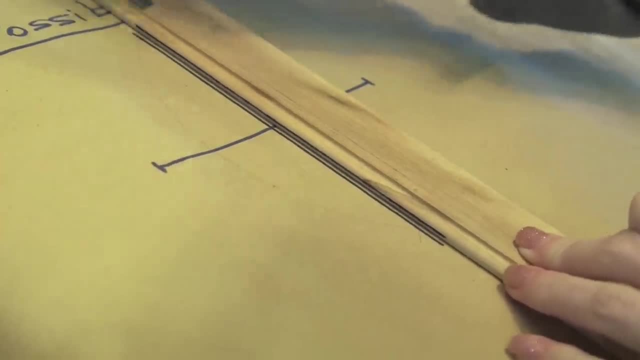 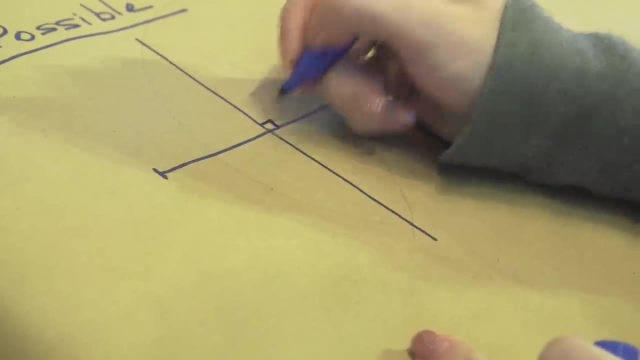 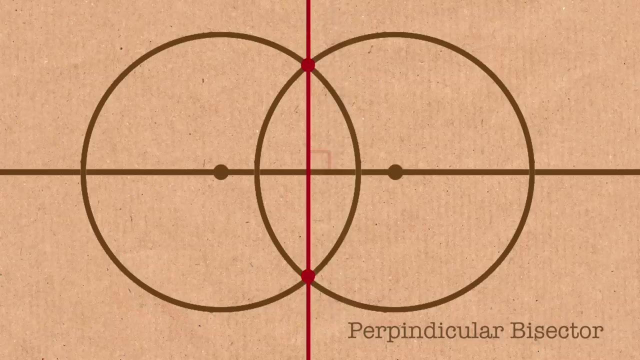 intersect, because I opened the compass Wide enough to be wider than half, And then this line is a perpendicular bisector of that. So why is that? I won't maybe show you all the proofs, but I will show you this one, If you connect all of these points. and what is this shape? 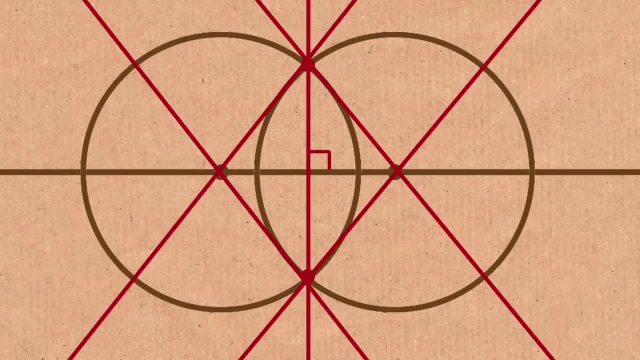 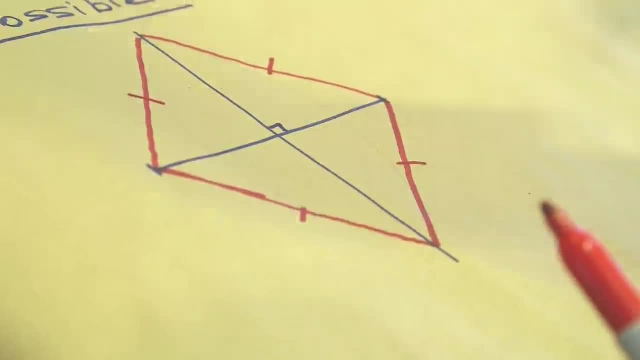 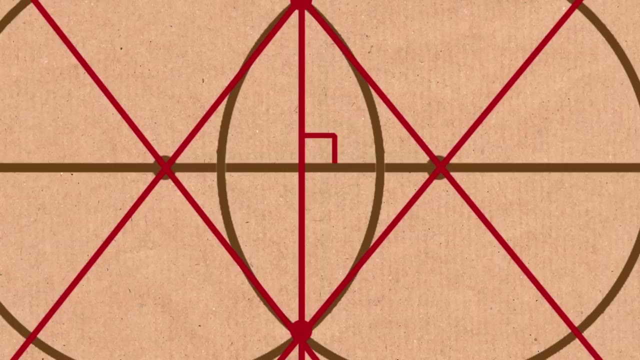 Well, all of these red lines are the radius of the circle, And those are all the same. They are all the same length because I kept the compass the same width the whole time, And so this shape is what's called a rhombus. One of the properties of the rhombus is that 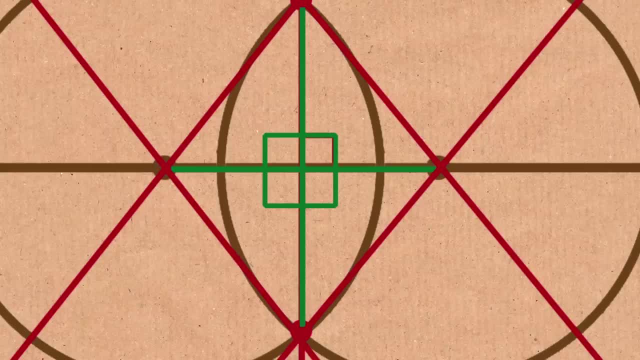 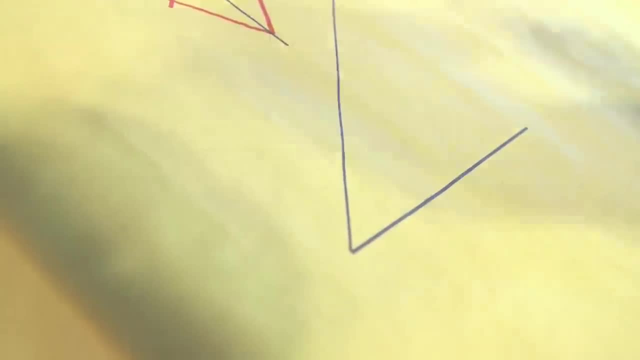 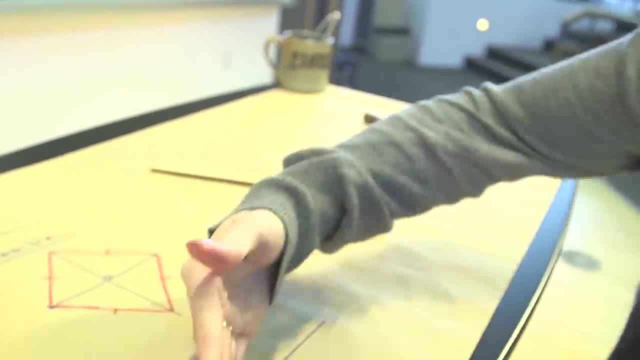 the two diagonals are perpendicular to each other and cut each other in half. Another thing you can do this is some angle. We don't know how big it is. We can't measure it because we don't have an angle measuring device. But whatever it is, I can bisect it, meaning I can construct a line. 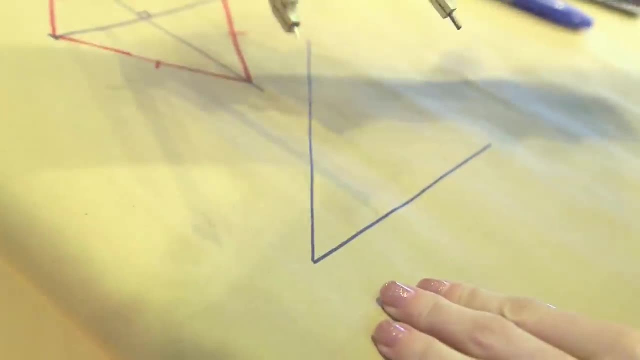 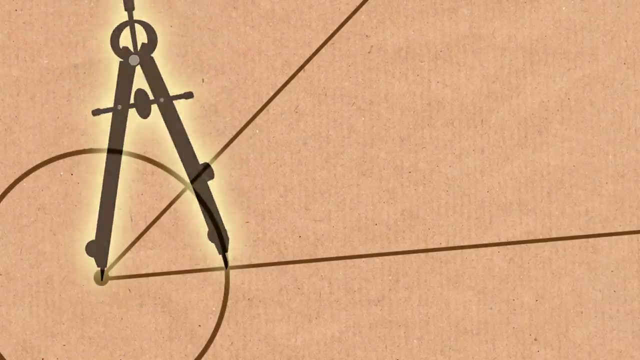 which is right in the middle of the circle, which is right in the middle of the circle, the middle. So how do we do that? We take the compass, open it to whatever width, doesn't matter, draw a circle arc and then, from where the circle arc intersects, 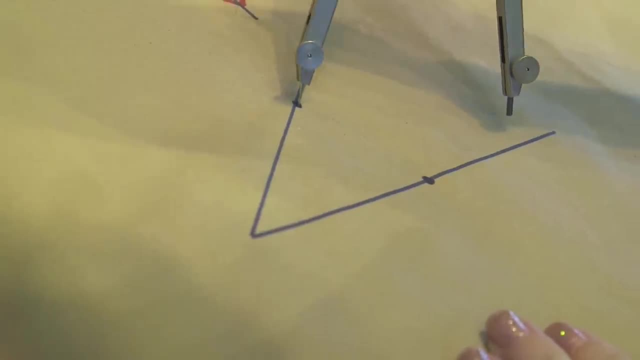 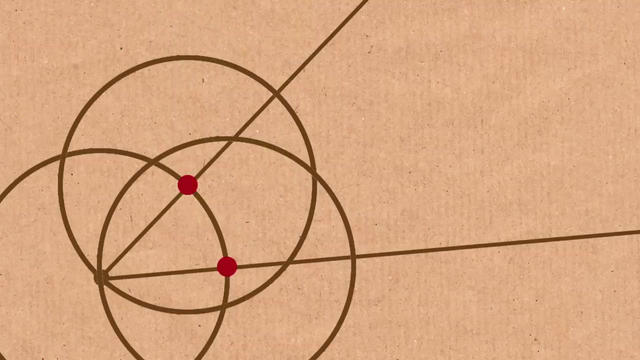 those two lines, we draw another two circle arcs, and these two have to be with the same radius as each other. And then, where those two intersect, we draw a line, and that line will bisect the angle, And again. so let me show you one. 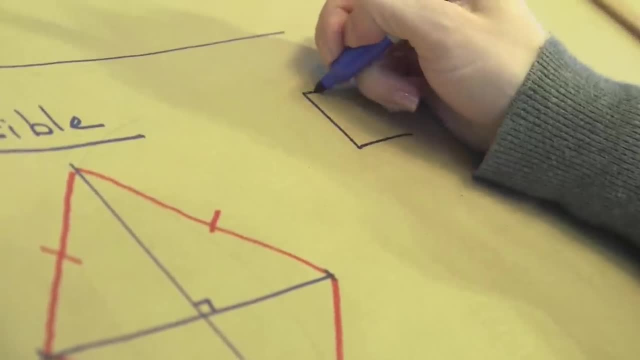 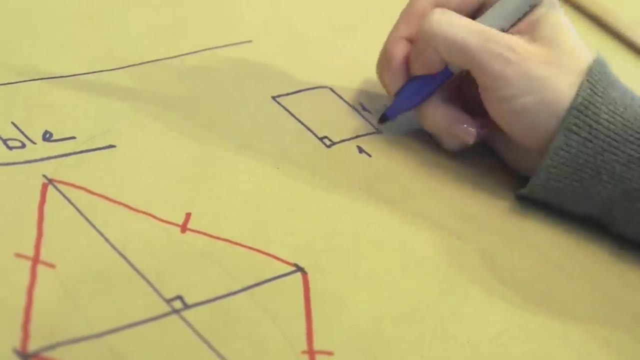 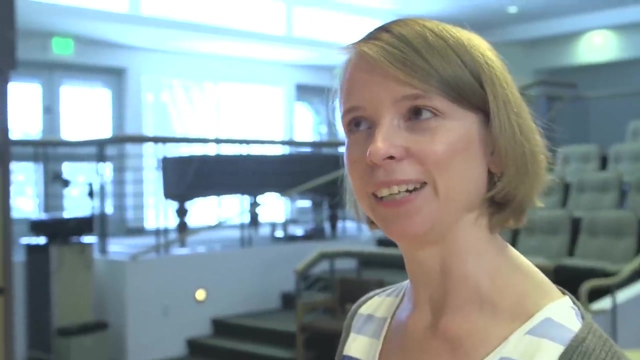 last trick that's possible. So suppose you are given a unit square and I tell you that every side is of length one and I ask whether you can double the square, meaning construct a square which has twice the area of this square. Okay so, 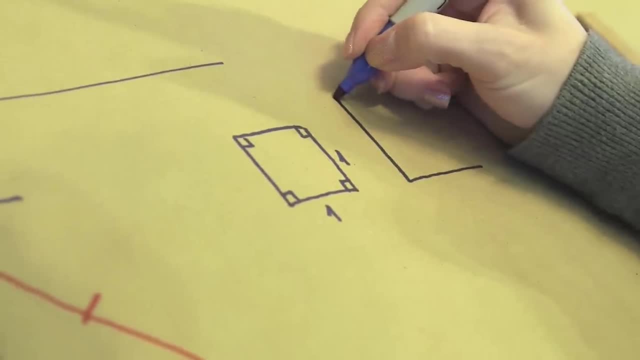 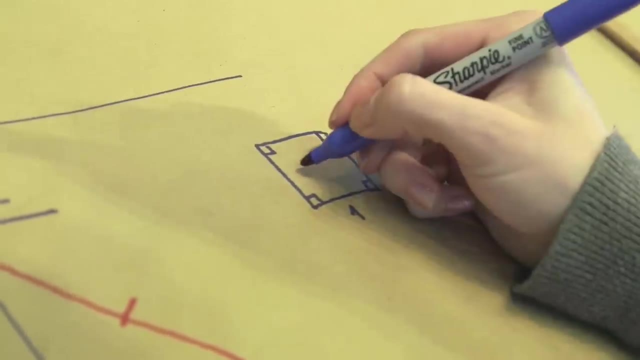 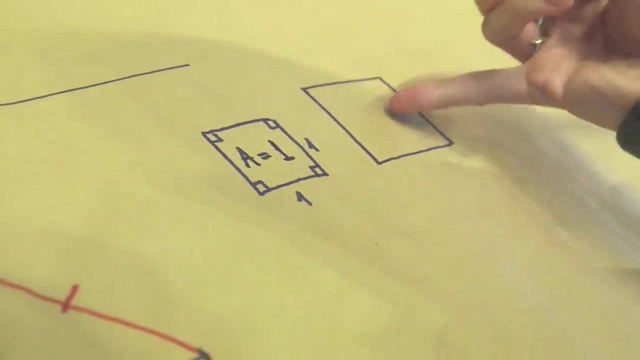 how would that go? Well, what we want is a square that has twice the area. Now, what's the area of this square? One One, because you get the area of the square by just multiplying the side lengths, So the area of this is one. so if this has twice the area, then the area of this is: 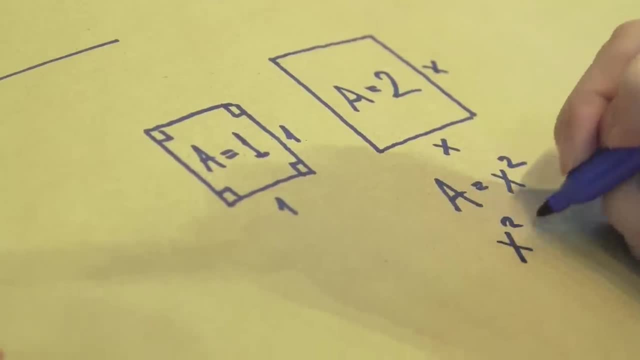 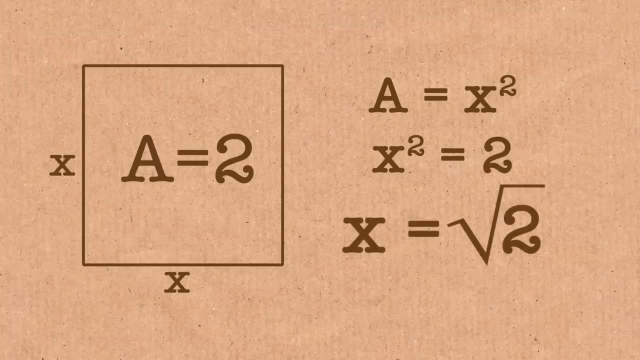 two, And that means that we know that x squared is two, and so we know that x is the square root of two. So how do we construct this square that's double the size? it comes down to having to construct a line. segment of length. 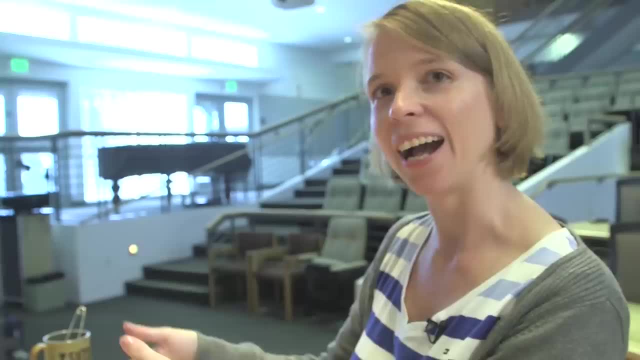 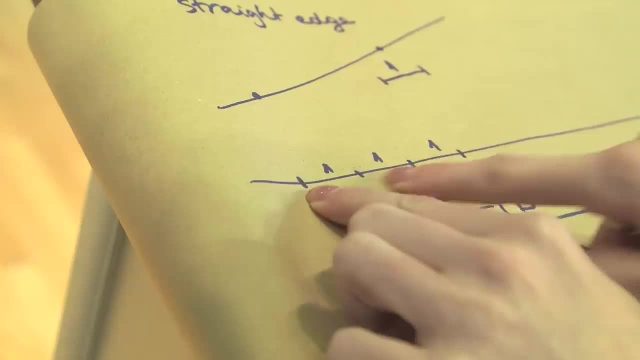 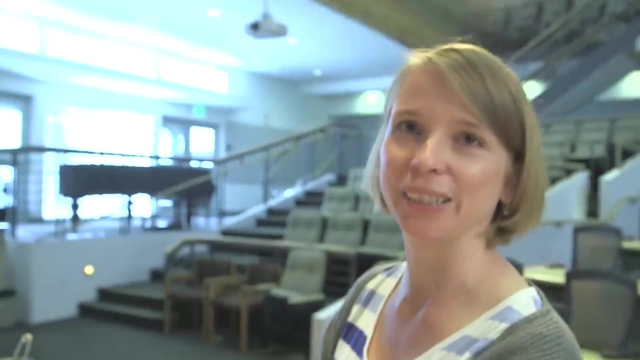 square root 2.. And this is where Euclid's kind of question starts to look more like your kind of question: Can you do a line segment of length 20?? Now his kind of question- can you do a square that's twice as big? comes down to a question which is our kind of question: can you do a line? 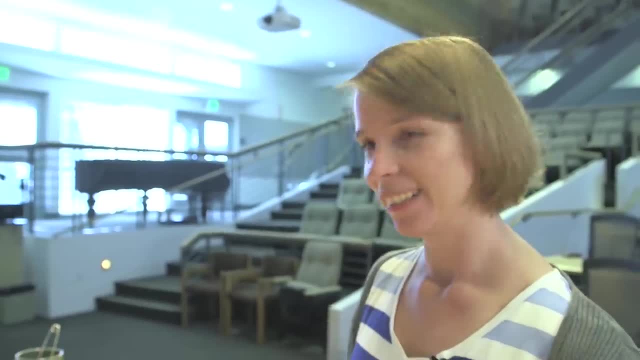 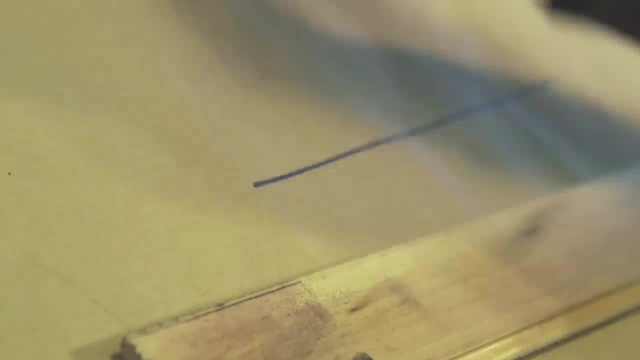 segment which is of length root 2? Can you do a line that's root 2 long? Yes, So how do you do that? You draw a line. Okay, now we want a line perpendicular to it, pretty much anywhere, And one way we know. 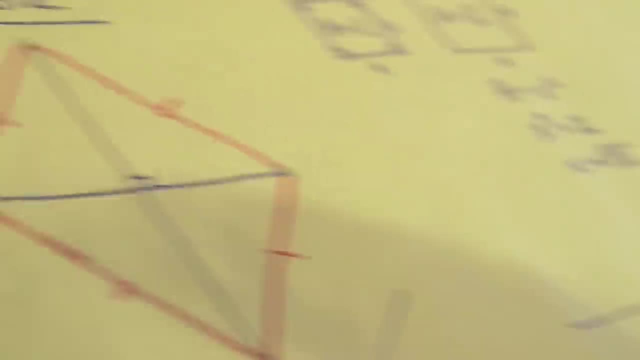 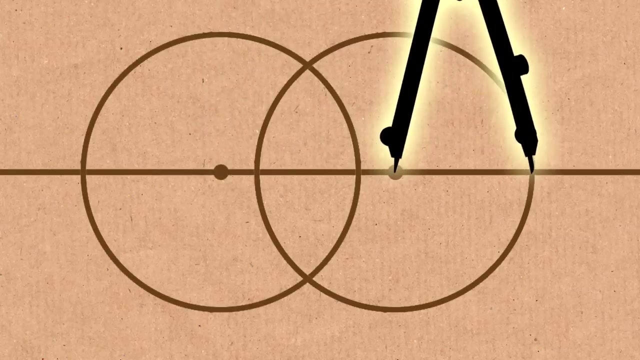 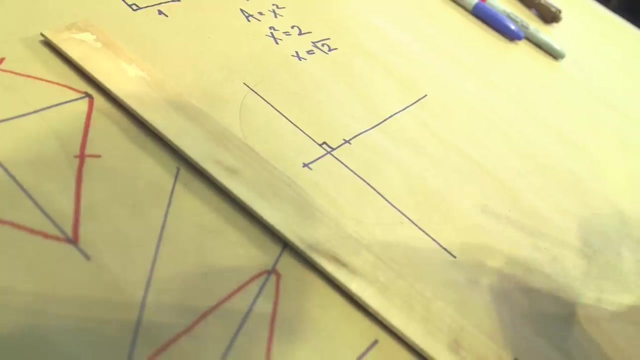 how to do that is we can construct perpendicular bisectors. So if I just pick two points, doesn't matter at all, There they are- And then I construct a perpendicular bisector to that little line segment, that will be a perpendicular line, And then we forget about those points, What happens if I take my compass? So I'm. 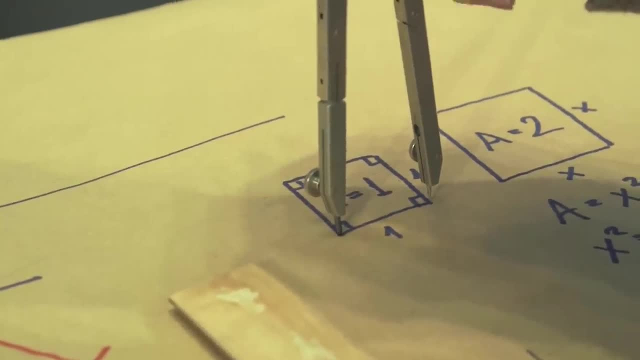 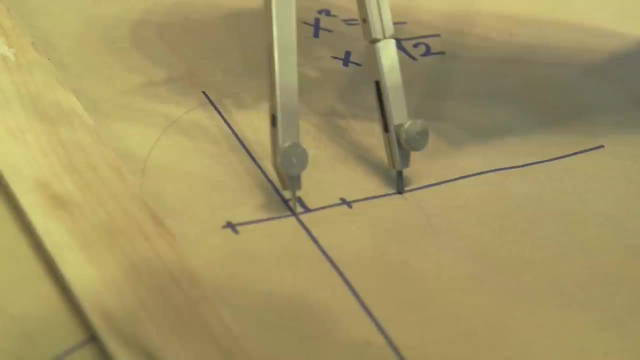 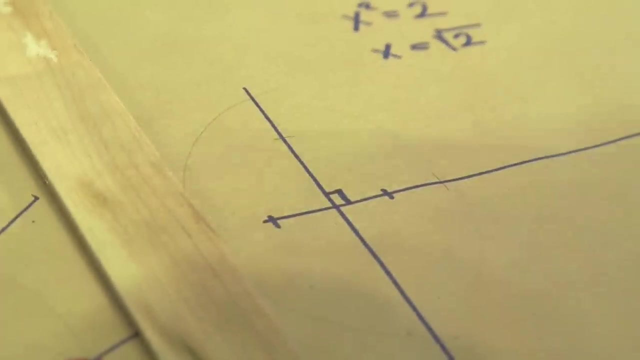 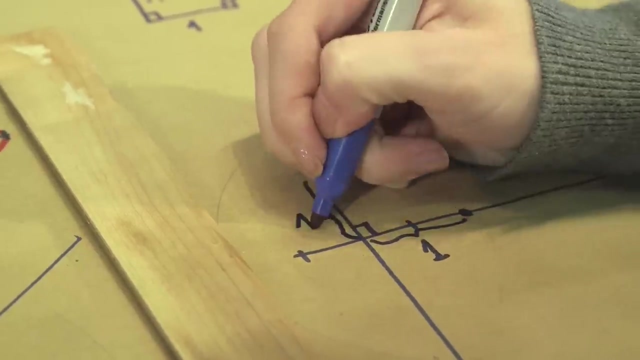 given this unit segment. That's the key. I know what length 1 is. And then, if I know what length 1 is, what happens if I put length 1 here and the length 1 here? I'll mark those. So this is 1, this is 1, can you guess what's next? 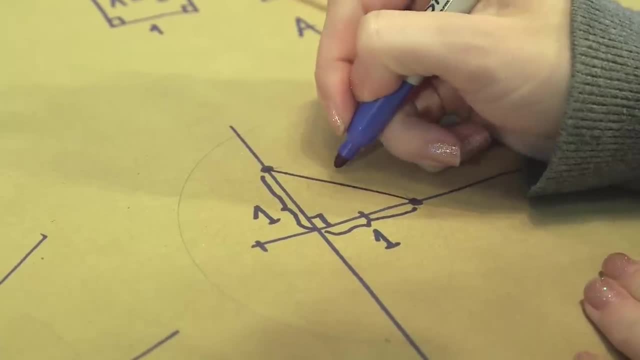 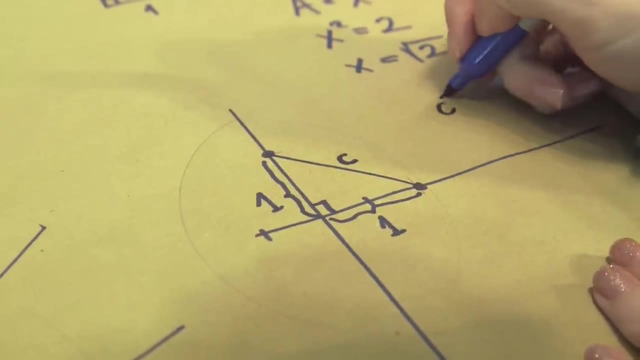 Yeah, you're gonna do a hypotenuse, Exactly. So this is a hypotenuse and you can use the Pythagorean theorem. so this is: if this is c, then c squared equals 1 squared plus 1 squared. so c squared is significance of one square. 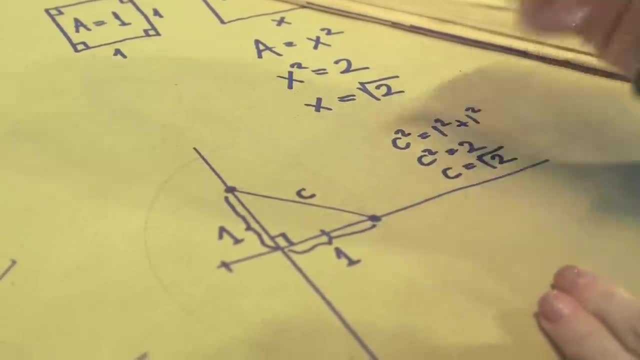 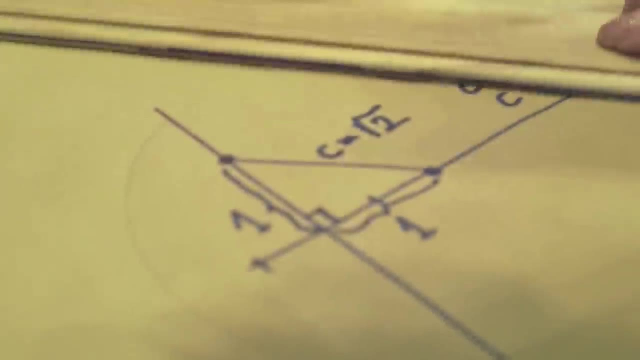 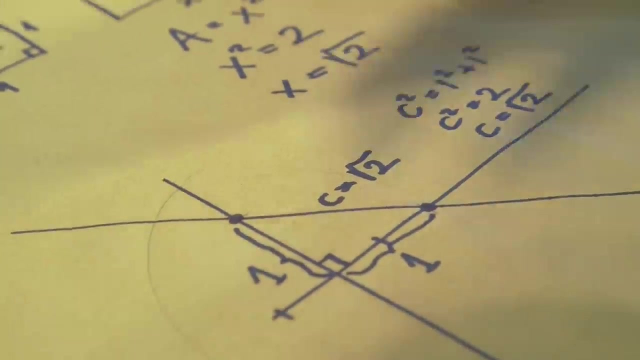 equals 2, and so c equals the root of 2.. To finish the job, well, you would have to make a square that has this as a side length, So let's just make it a bit longer. We want perpendicular to it here and perpendicular to it here, and we know. 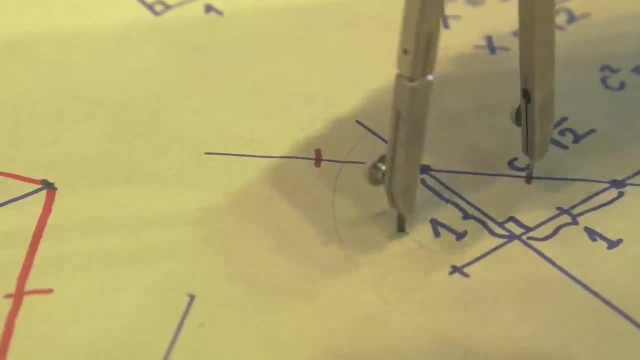 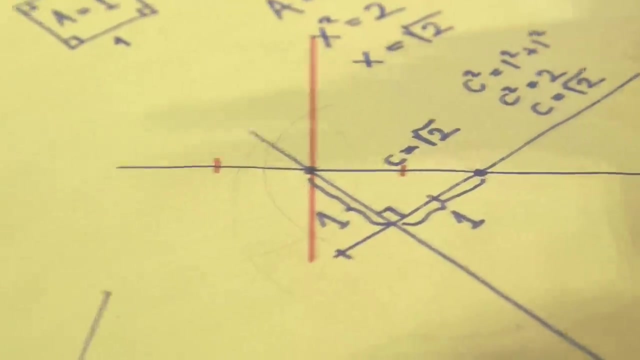 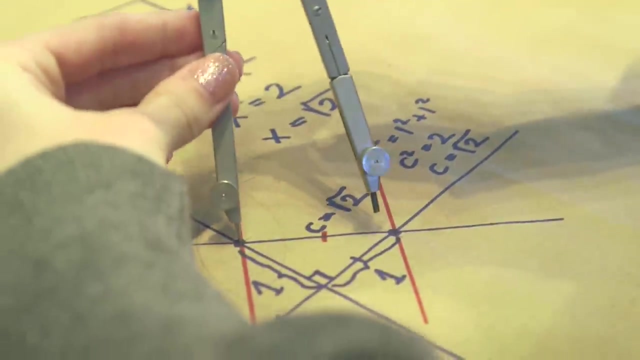 how to do perpendiculars. Draw a circle arc, draw another circle arc, okay, And then you'll believe me that I can do that on the other side as well. Yes, We have now three sides of the square. we just have to measure the side length. So put this: 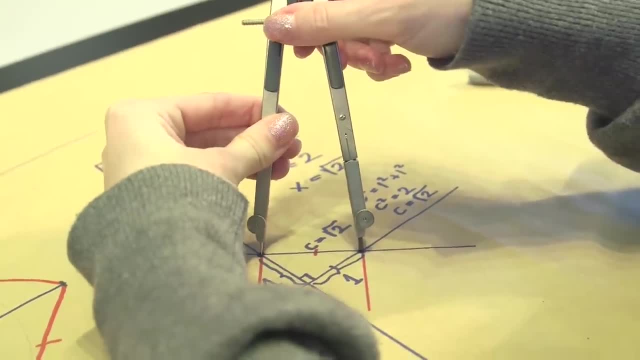 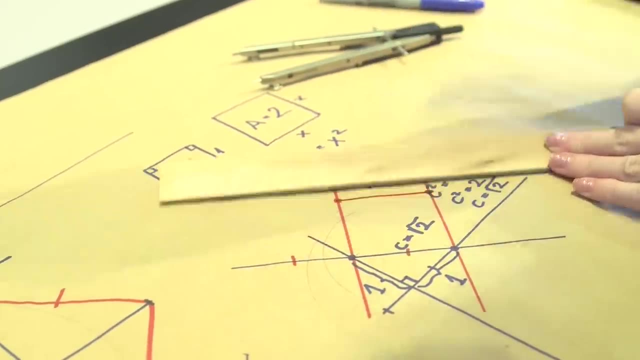 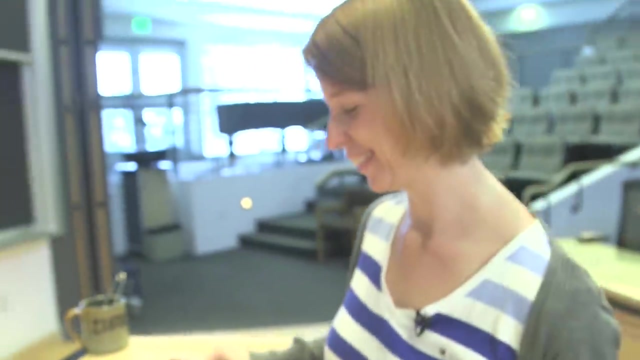 in here. This is the length root 2, so I measure it on that side And then I measure it on that side, the whole square. Well done, So that is job done. Yep, So you can double a square. A question: 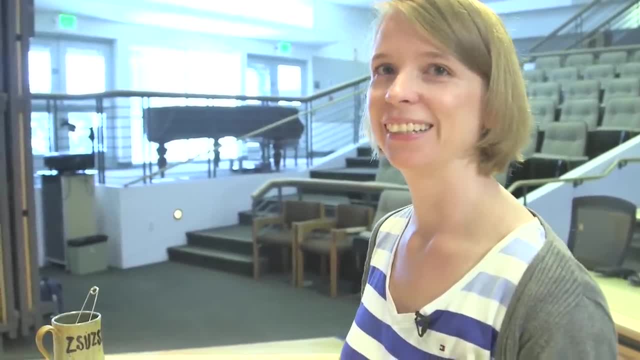 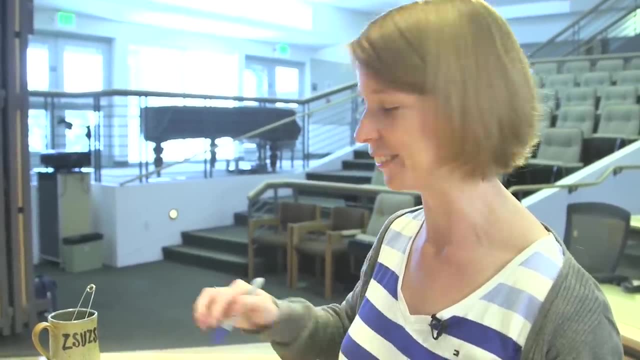 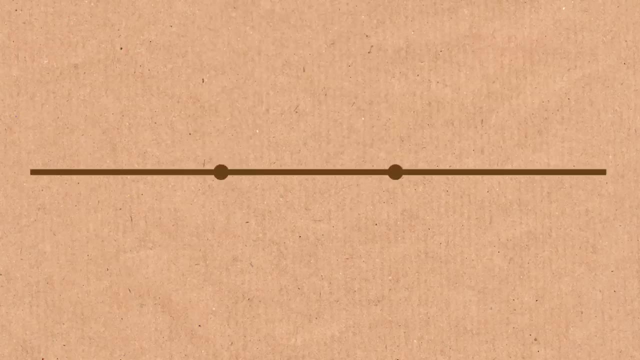 that you could try figuring out is how to triple a square. So it's very similar to this, but it involves a little bit of extra trickery. It's a fun problem to think about. What's the first thing I showed you? It's how to bisect a. 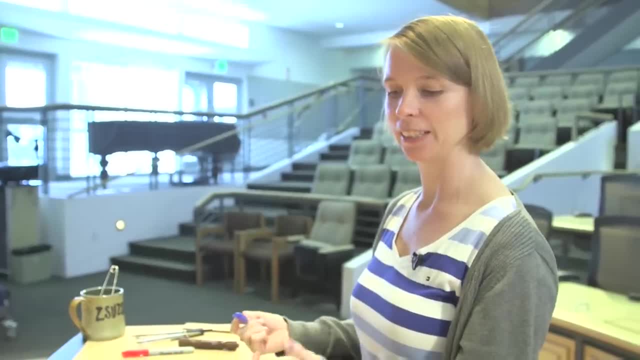 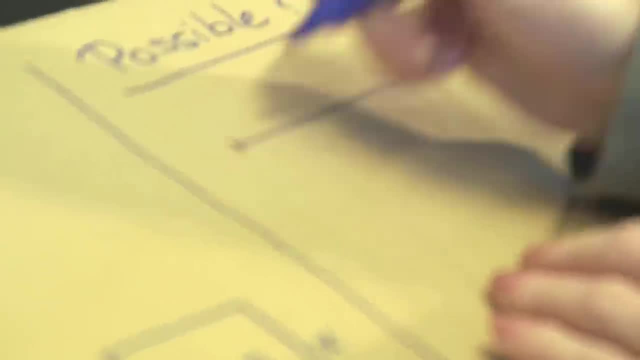 segment. So, instead of asking how to bisect a segment, I could ask: can you trisect a segment? So can you cut a segment into three equal parts, as opposed to two equal parts? The answer to this is still yes, and it's actually. 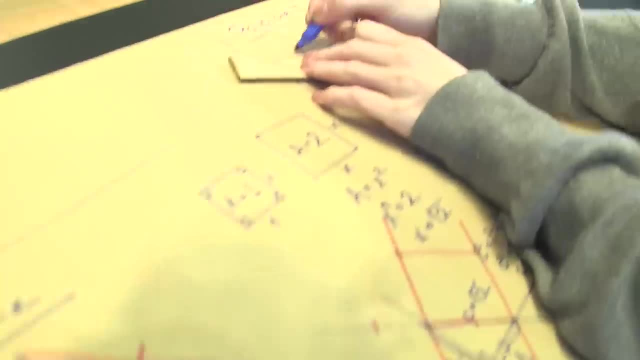 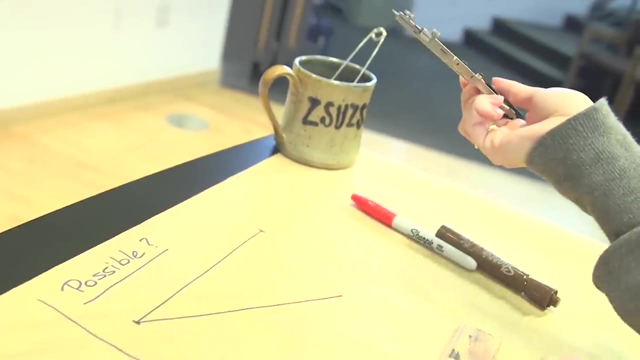 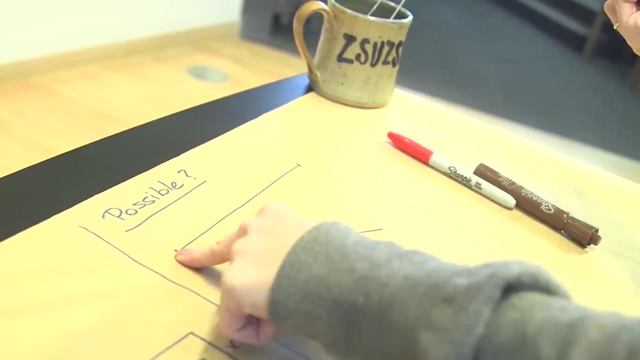 pretty simple. I won't do all the perpendiculars properly, because now you believe me that I can construct perpendiculars, so I'll just do it the shortcut way. So open your compass to any length you want. Put another line which starts at the same point as the light segment, What the angle is. 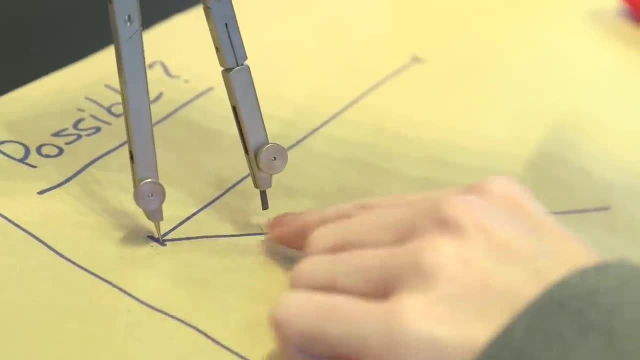 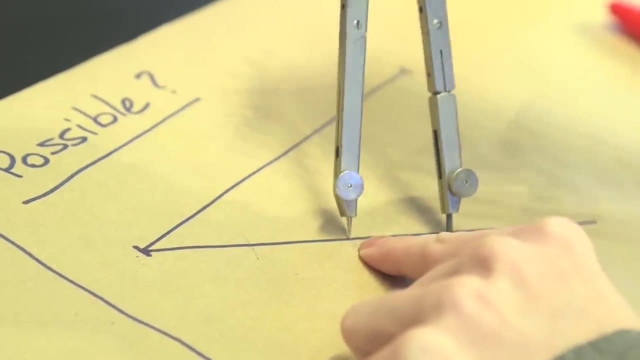 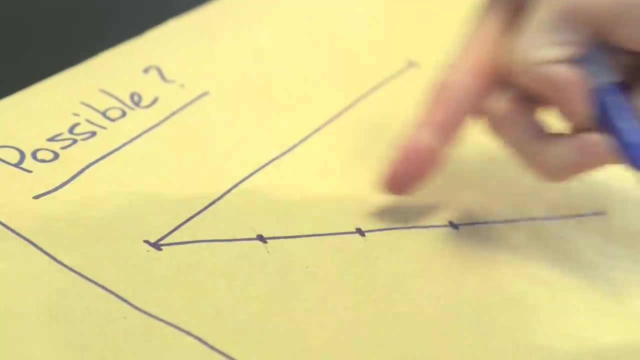 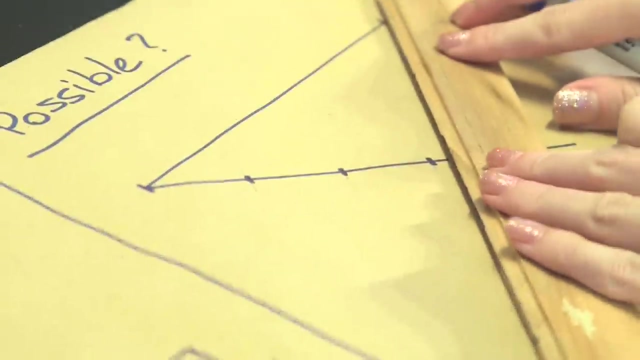 doesn't matter whatsoever. Put your compass at the end and measure that This, whatever length, doesn't matter, One times, two times, three times. so now, on this other side, I have constructed a line segment which is trisected by design, and then connect these two ends and then, from this point, draw a parallel. 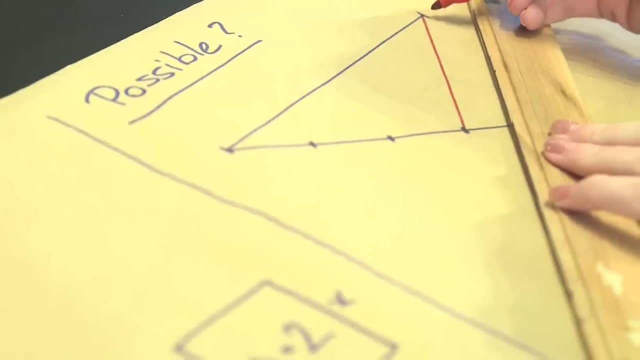 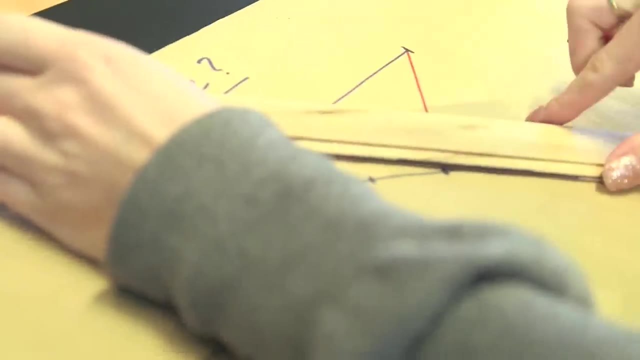 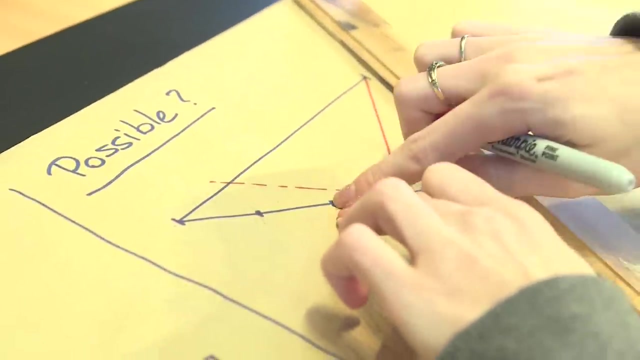 to this red line. Now, I haven't told you how to draw, but a parallel is what's perpendicular to a perpendicular. So what you would do is you would draw a perpendicular to that red line here and then you would construct a perpendicular from this point to that. 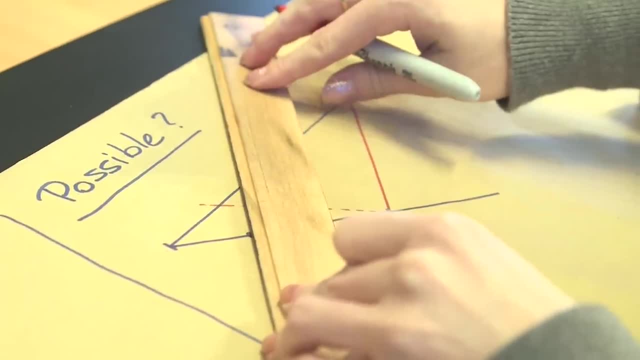 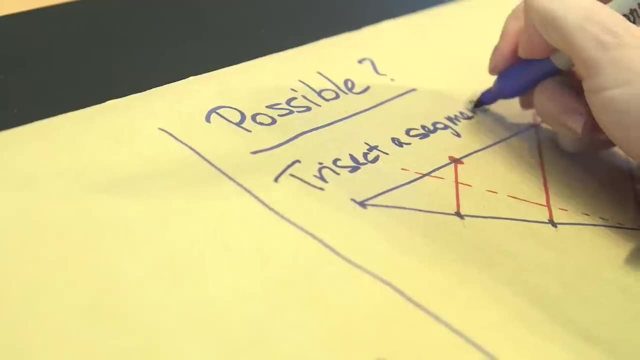 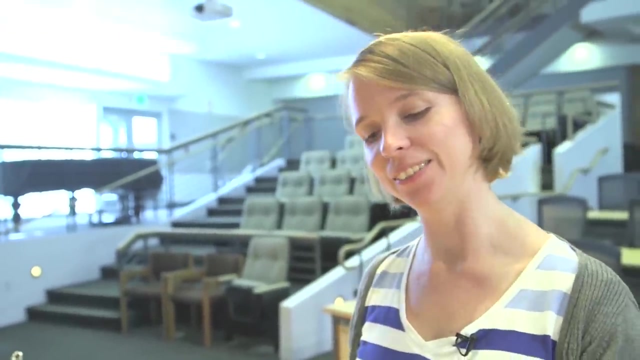 and that would be parallel. And then another one from over here, And magic, where it intersects, trisects that original line. So the next thing, next natural question: I showed you how to bisect an angle. Can you trisect an angle? 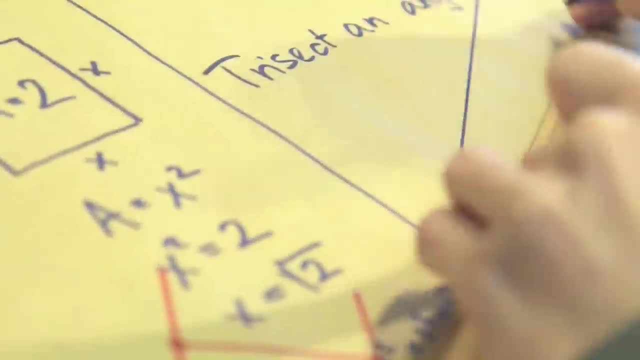 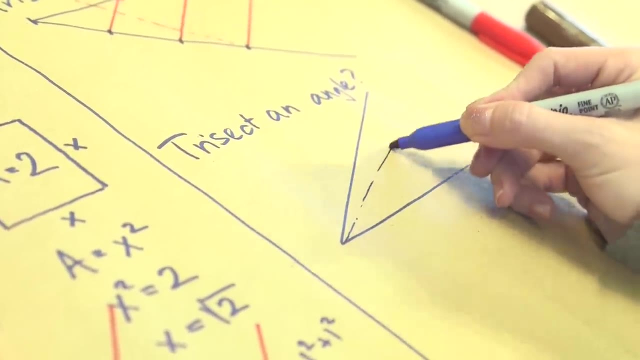 So I give you some angle. You don't know what the measure is, because you don't have a measuring device, And you come up with a construction which will result in two lines which divide that angle in three equal parts. Well, based on everything, 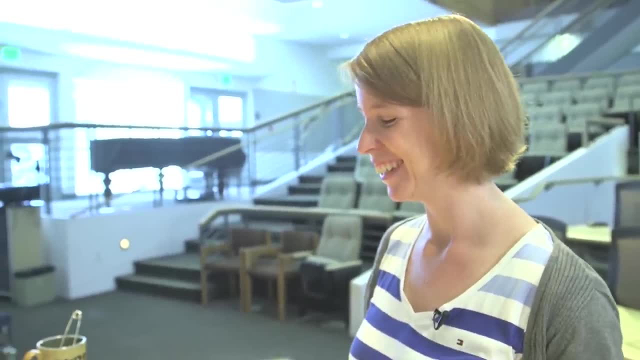 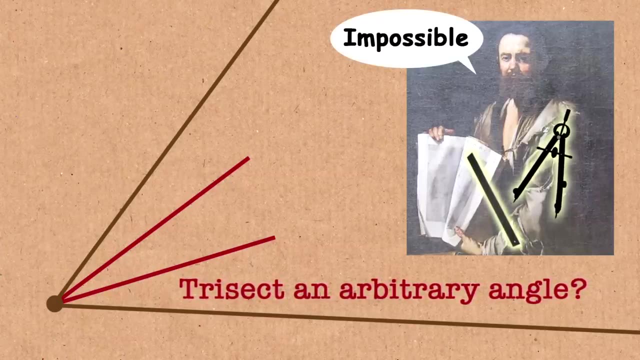 you've shown me so far, I would have said yes, Well, Euclid couldn't. And then for about 2000 years, people thought about this problem. Before I tell you the answer, let me give you another problem. So I told you that you can triple a square. 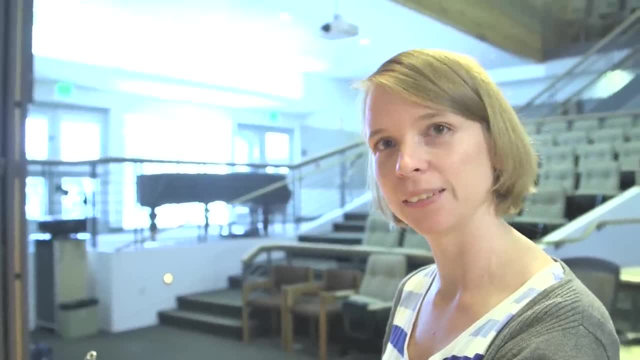 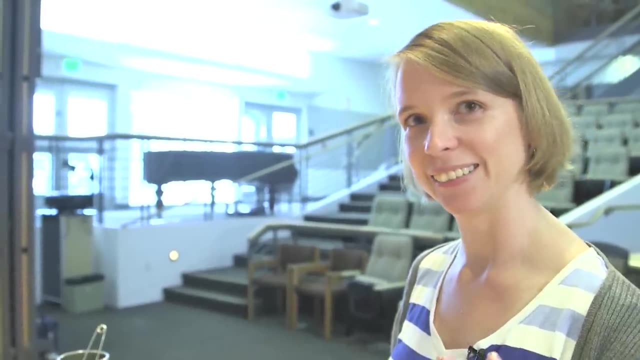 That's one kind of generalization of the problem of doubling a square. It's going up in the ratio by which you want to multiply. Well, you could also try going up in dimension, So a square is a two-dimensional thing. So instead of doubling a square, 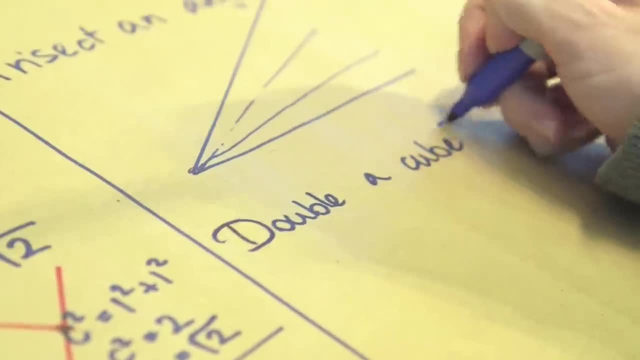 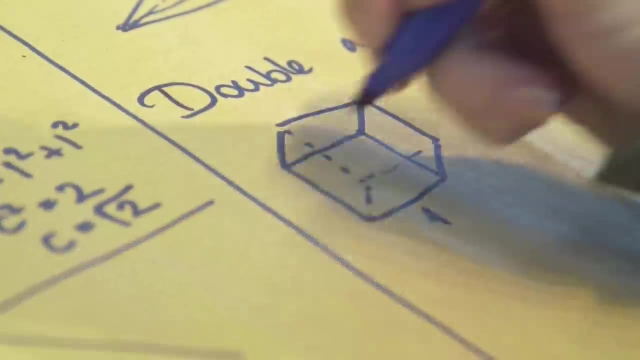 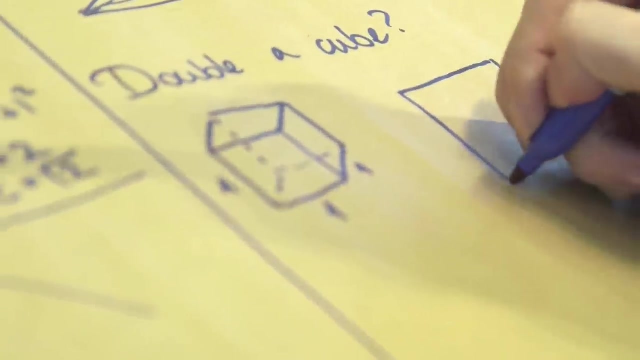 you can ask about doubling a cube. So what does that mean? Well, you're given a unit cube, meaning a cube whose sides are all length one, And what you want to try to figure out is how to construct another cube which has twice the volume. 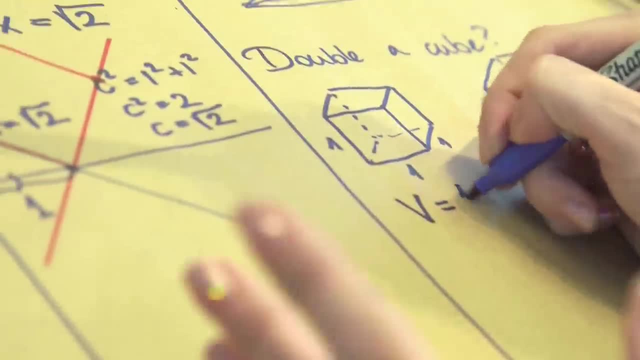 Now, what's the volume of the unit? cube One: One. because you get the volume of a cube One. One because you get the volume of a cube One. because you get the volume of a cube Three. because you get the volume of a cube. 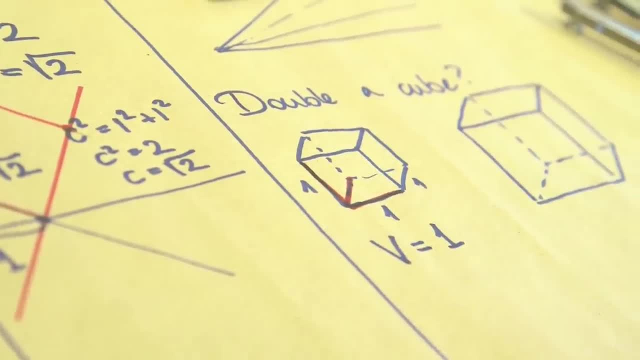 So you get the volume of a cube by multiplying this side length, this side length and this side length, which are all the same because it's a cube. So that's one times one times one is one. So if we doubled it, 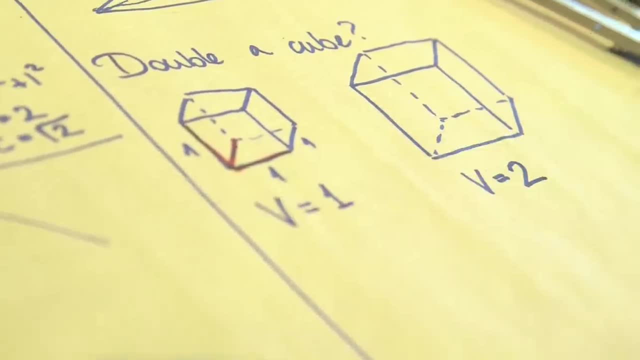 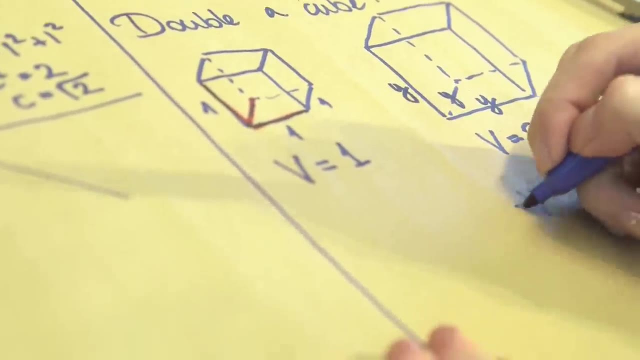 then the volume of the new one would be two. So we don't know what the side length is, but we can figure it out. If the side length is y, then I know that the volume which is two is y times y times y. 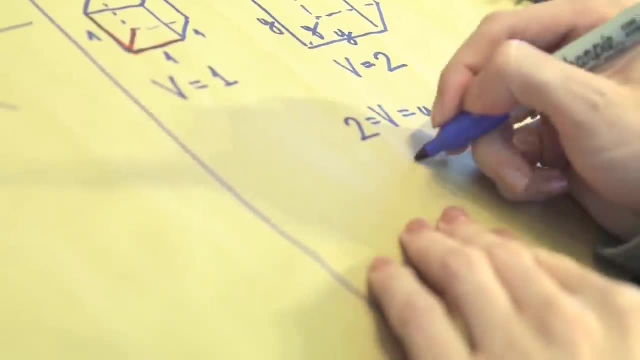 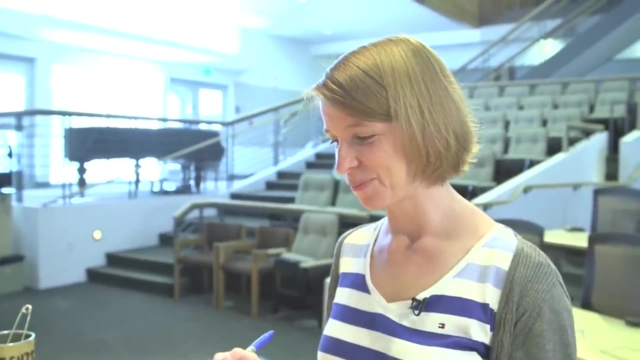 so it's y cubed. Well, to get y we have to take the cube root. So y equals the cube root of two. can we do a cube root of two? can you do cube roots using a compass and a straight edge? well, who knows? euclid couldn't. and then people thought about it for two thousand years, so both. 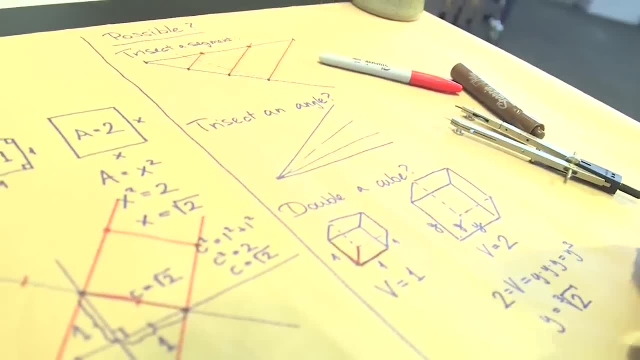 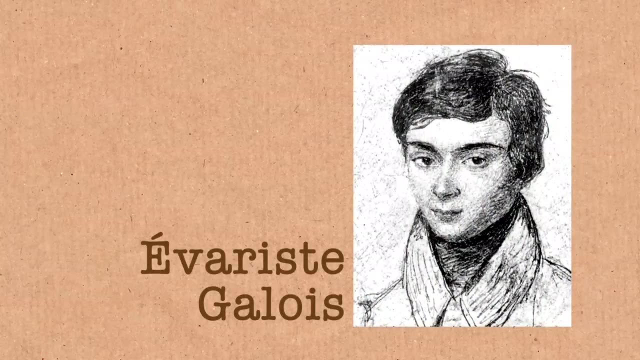 of these problems euclid couldn't crack. both of them euclid couldn't crack. people were very curious about them and many, many smart people thought about them. and then in the early 1800s came along this ingenious guy called galois. he died at age 19 in a duel, but before that he 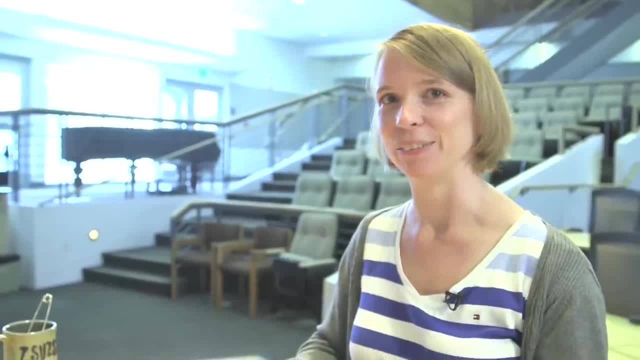 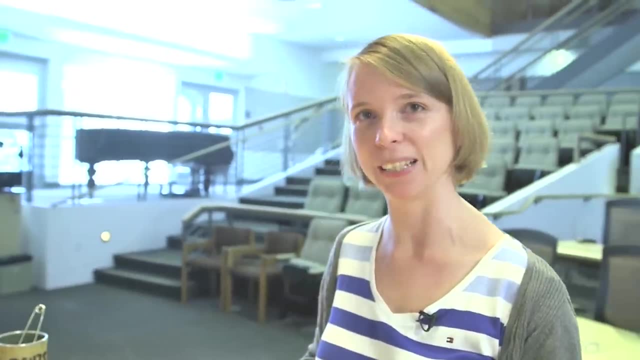 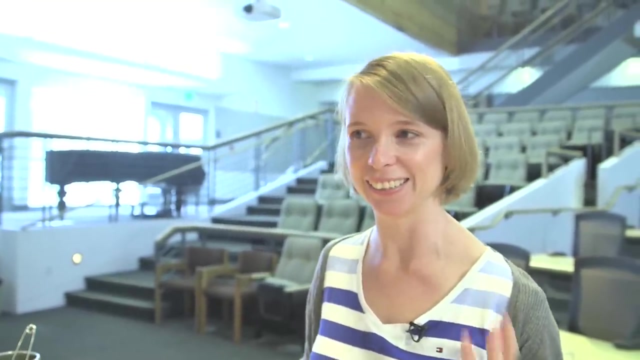 essentially revolutionized, uh, algebra before he was 19, before he was 19, yeah, wow. so this theory, galois theory that he came up with um, is now, if you're in any math program in university, you're taught this in your, say, fourth year of undergraduate or first year of graduate studies. i hope they 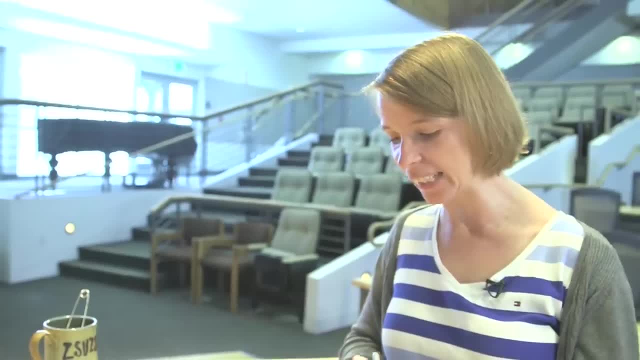 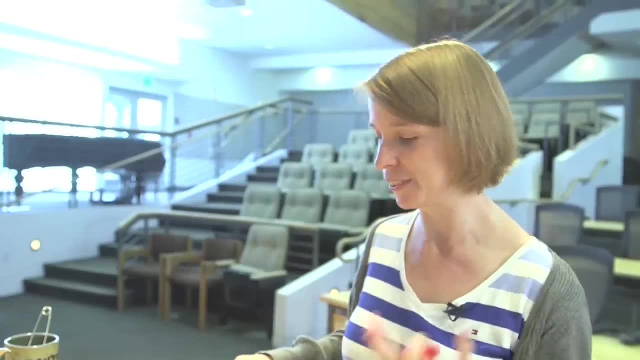 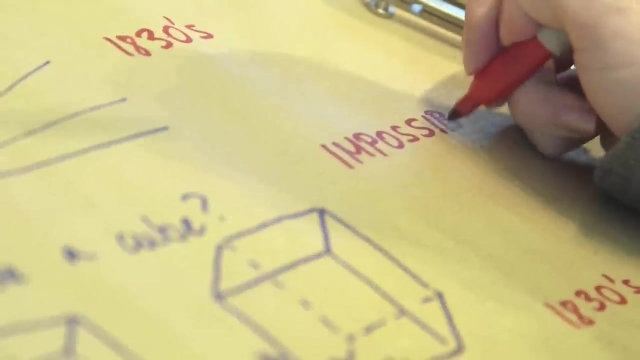 also teach you not to have duels. so that gave people the tools to eventually crack these problems, and they were. they were well not solved, but it was proven in the 1830s that both of these are impossible, and the guy who proved both of these call is called pierre oneself, and you can see why they. 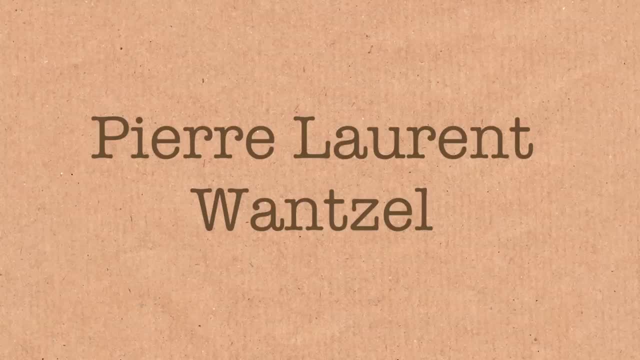 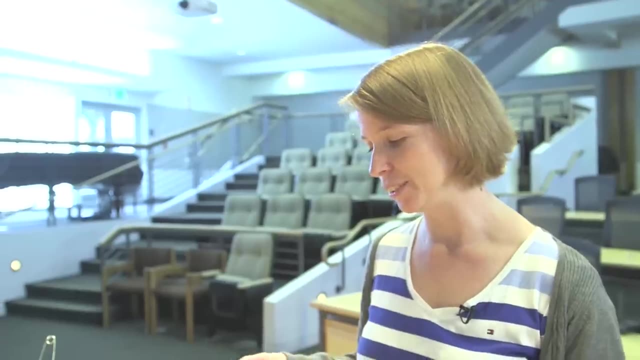 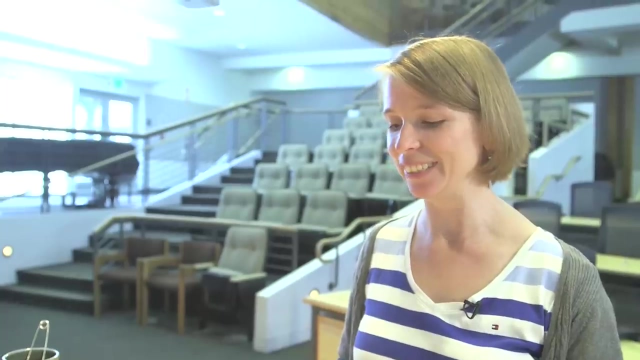 were so much harder, because when something is solvable, all you need to do is come up with a solution. these solutions stay are tricky but they are not that hard. but to solve that something is impossible, that's to prove that something is impossible, that's hard because you can't. you know. saying that, i thought. 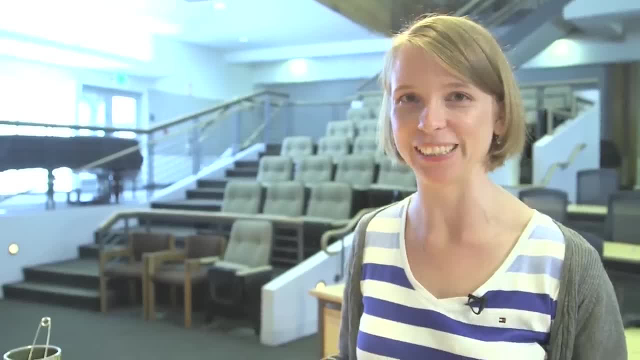 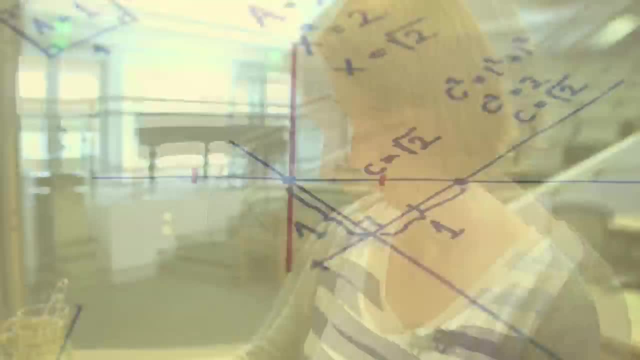 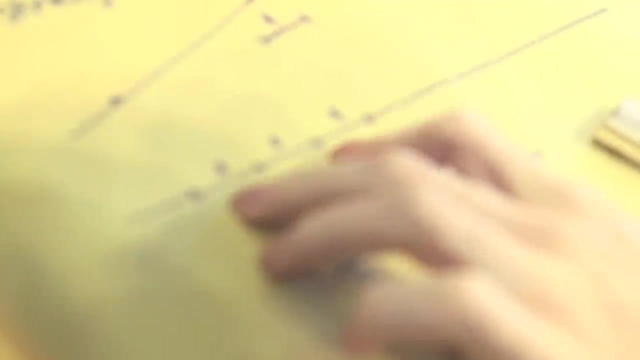 about it for 10 years and couldn't do. it is not a proof. maybe you're just not smart enough, so. so you have to come up with something explicit that proves that they are absolutely impossible. and what it came down to is exactly your kind of question. what kind of lengths? 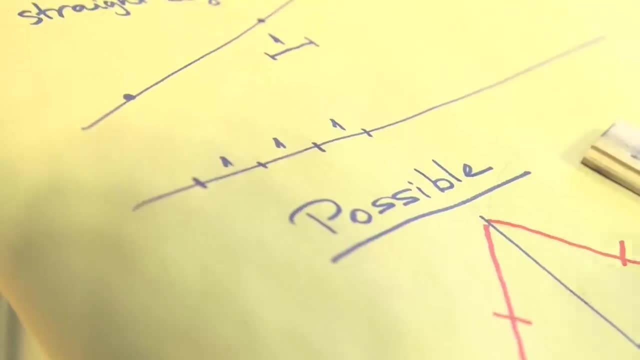 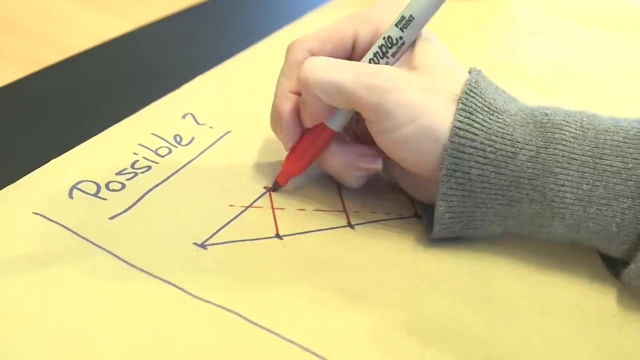 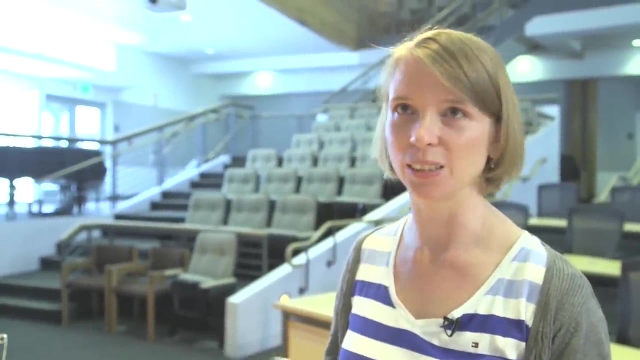 you construct if you're given a unit segment. so i, for example, i showed you how to do square root 2, i showed you how to do 3, i show you how to do one third. it turns out that you can do all numbers that just involve fractions and square roots and addition and subtraction. but there's a problem. 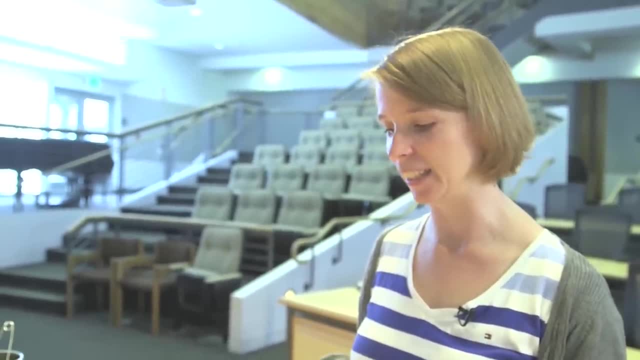 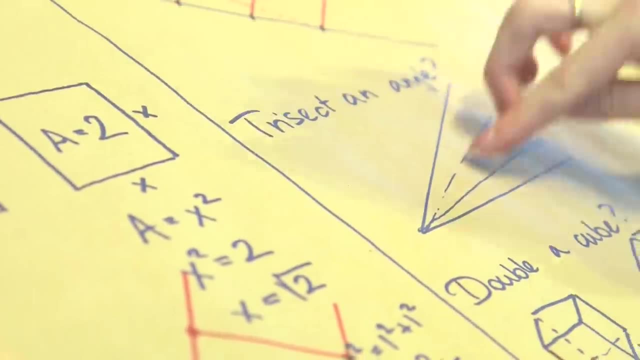 with cube roots. so what this guy proved it is that you will never be able to do cube roots, and that can also be used to crack this problem, because trisecting an angle somehow comes down to cube roots through trigonometry. so cube roots are the 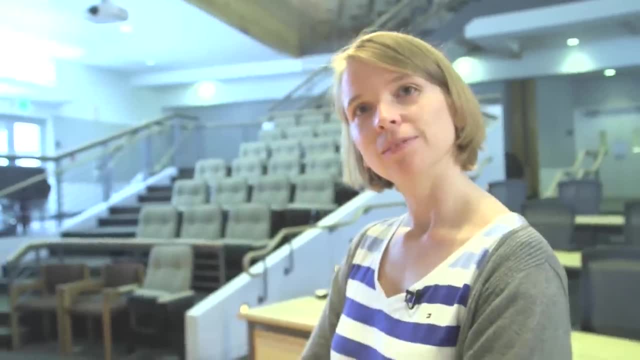 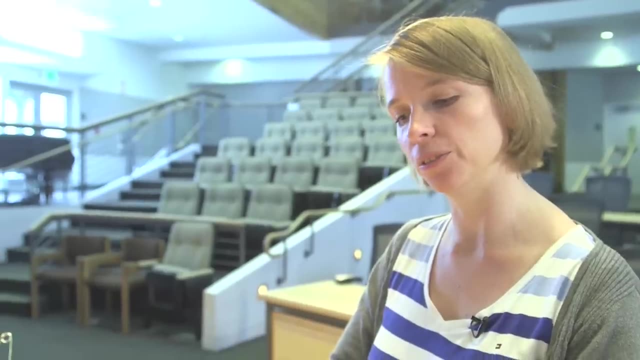 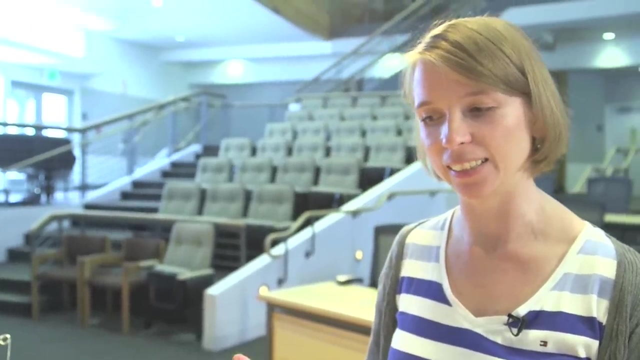 problem. cube roots are the big problem, but the same question applies: how do you prove you can't do cube roots? how do you prove that you can do cube roots? that's a very good question. what do you use to translate from geometry to numbers is the main question, and the answer is analytic.